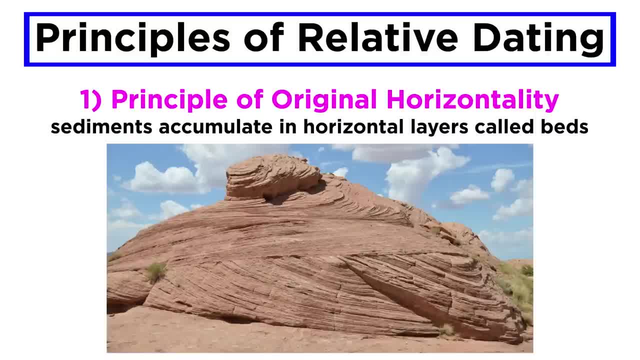 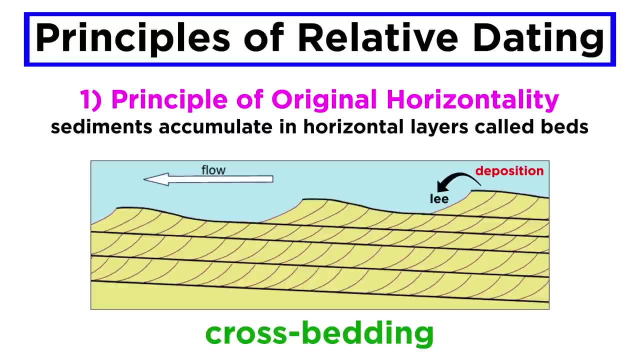 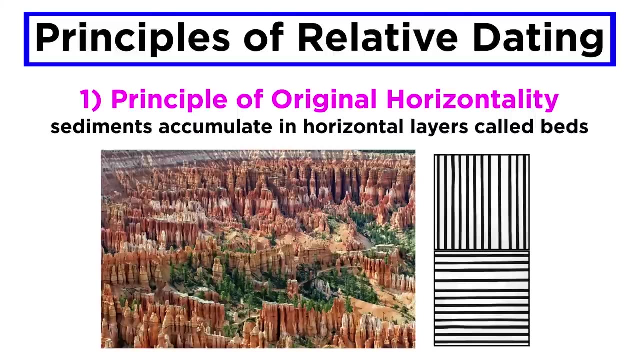 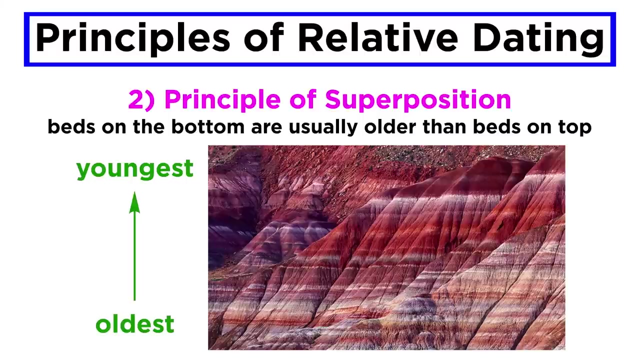 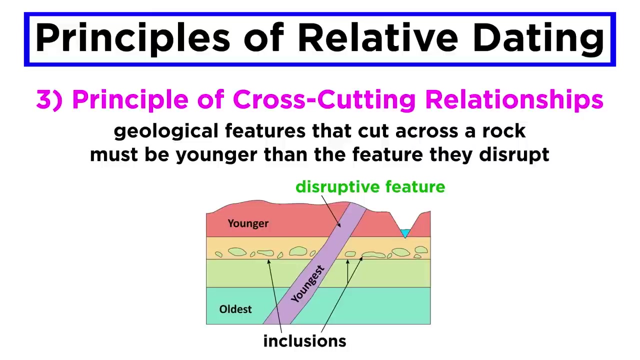 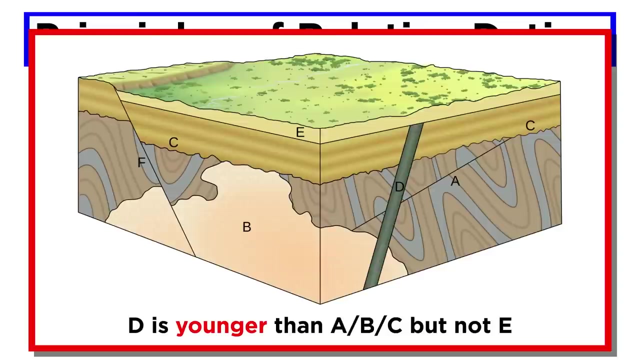 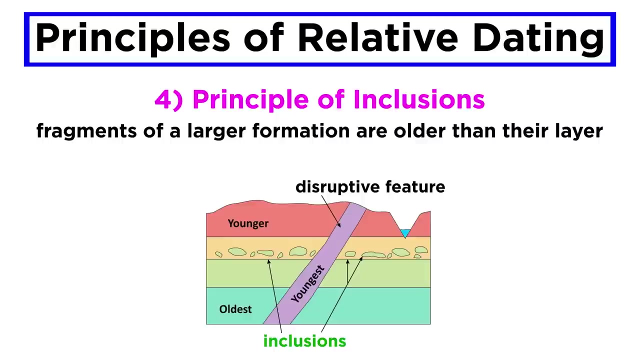 layer are called bed layers. The classification of sediment in the horizontal layers represents dunes, may be inclined as much as 35 degrees. This is called crossbedding. In crossbedded sedimentary rocks, the sediment is deposited in sets, at the angle of repose, on the lee side of dunes and ripples, which explains their inclination. In addition, only sand-sized sediment can form crossbeds. Say for example that you find an outcrop with a horizontally layered siltstone on top of a vertically layered siltstone. When you apply the principle of original horizontality, you realize that there was a large time gap between deposition of the horizontal and vertical formations. The principle of superposition states that, unless tectonic forces have overturned the outcrop, beds on the bottom are usually older than beds on top. The principle of crosscutting relationships states that any geological feature which cuts across the surface of a rock is a crosscutting relationship. The principle of crosscutting relationships states that any geological feature which cuts across a rock must be younger than the feature it disrupts. So, if an igneous intrusion is found cutting through a sandstone, the intrusion must be younger than the sandstone it cuts through. The principle of inclusions states that any rock fragments that are part of a larger formation must be older than the 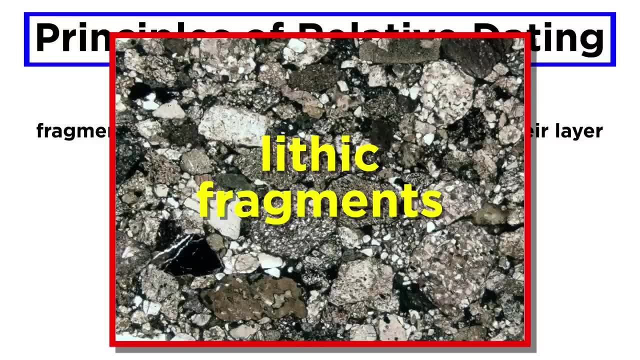 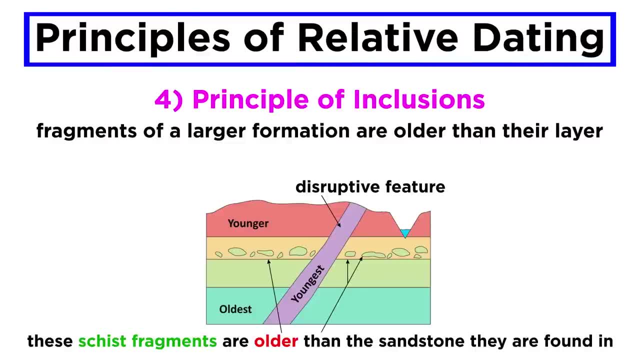 formation they are a part of. For example, lithic fragments, which are pieces of a pre-existing rock, are common types of grains in sedimentary rocks, so if you find a class of schist in a sandstone, the schist must be older than the sandstone it is a part of. 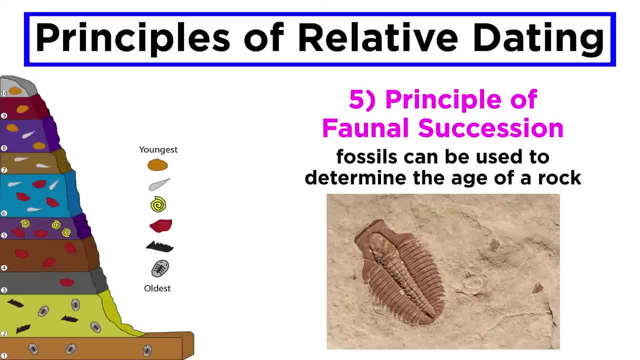 The principle of faunal succession states that there is a historical order in which organisms evolved over time, and that certain specific fossils can be used to determine a rock's age. 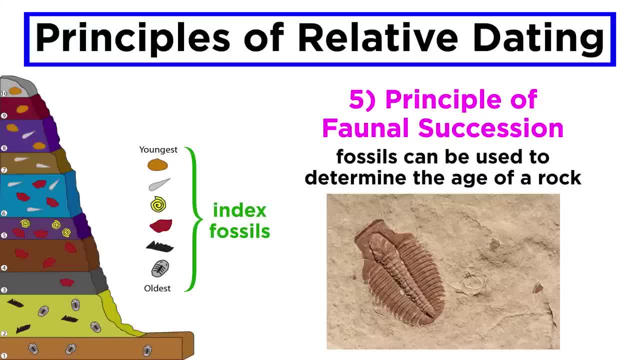 Organisms that only existed for a short period of Earth's history are most useful for this, and their fossils are called index fossils. For example, if you find a trilobite fossil in a bed, then it must have been deposited in the soil to form a new rock. However, if you find a trilobite 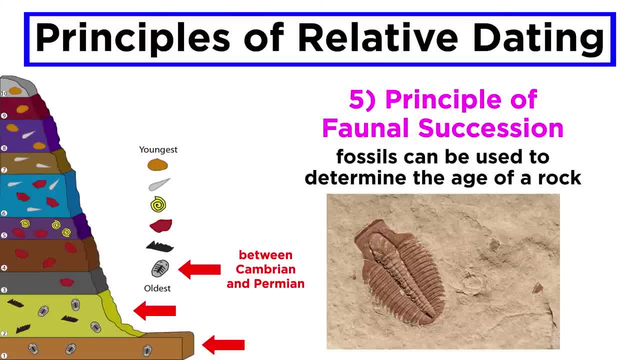 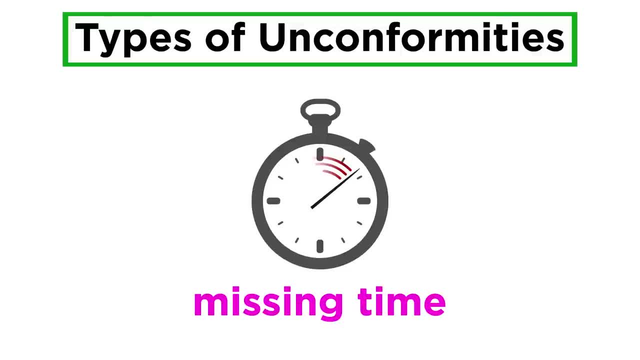 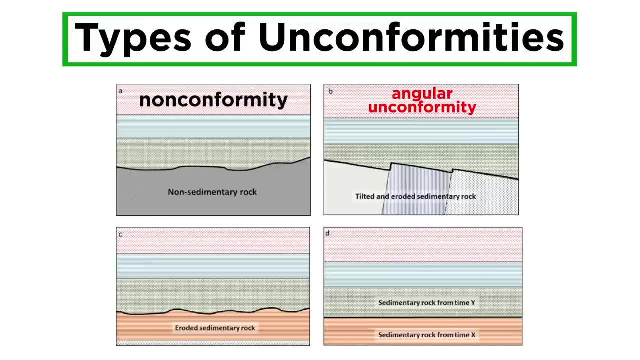 between the Cambrian and Permian periods. Another useful concept for qualitatively dating rocks is that of missing time, or gaps in the rock record called unconformities. There are four types of unconformities. A nonconformity, an angular unconformity, a disconformity, 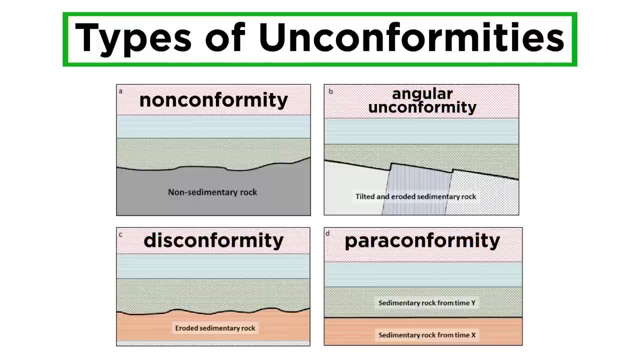 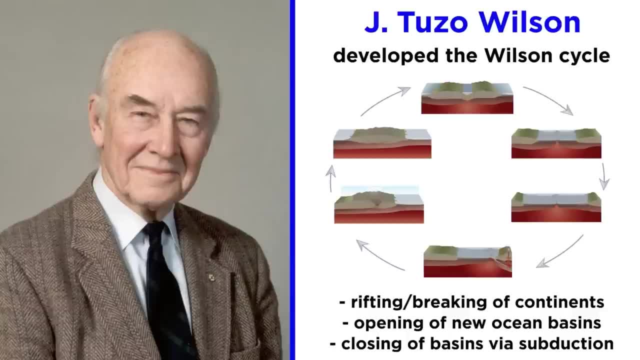 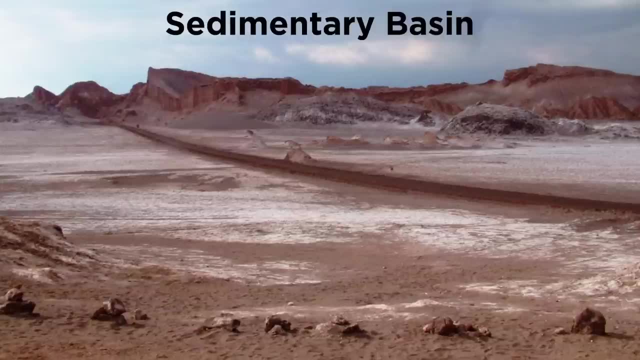 and a paraconformity, all of which represent missing time. But what exactly is meant by missing time? Recall the Wilson cycle from a previous tutorial and the ways that geologic environments change over time. For example, during one period, an area may be part of a sedimentary basin, but then get uplifted a hundred million years later during an orogeny, transforming the 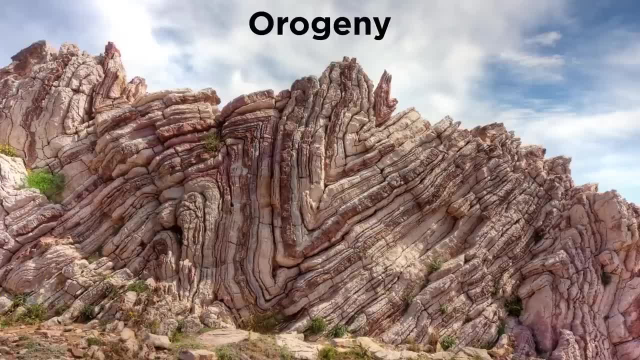 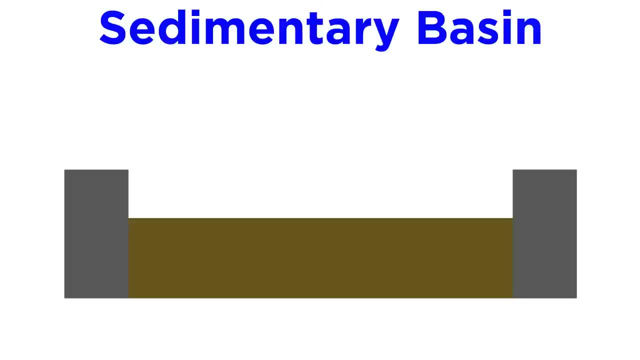 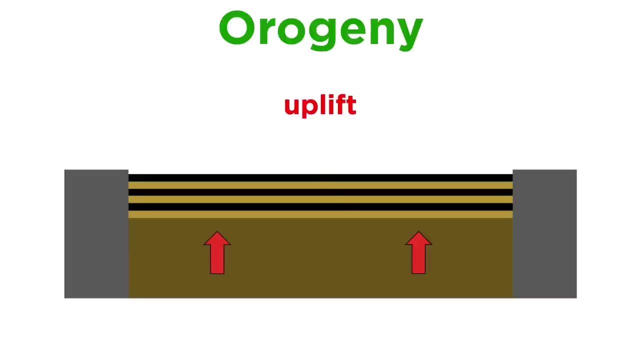 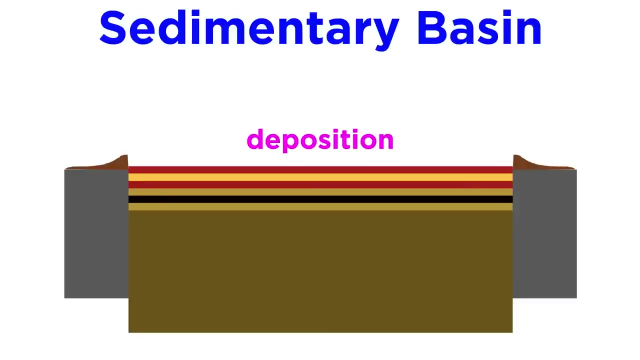 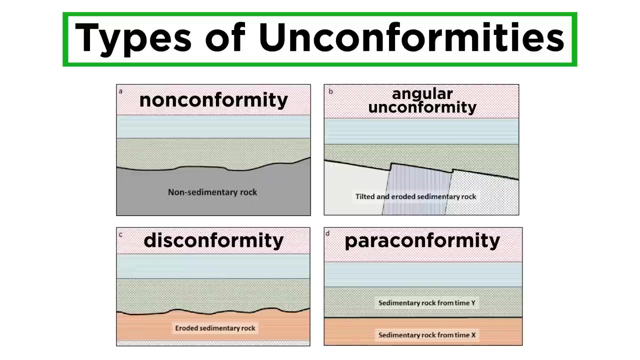 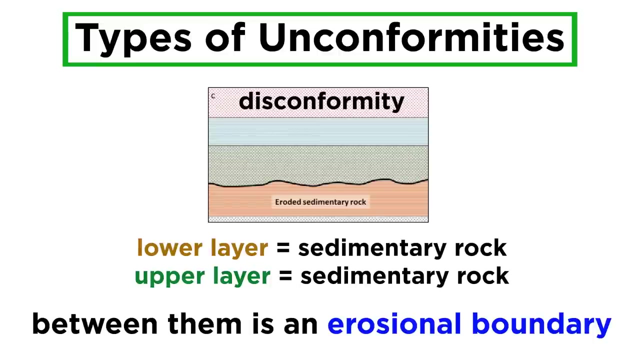 once sedimentary environment into an erosional environment, and then after another 100 million years, it could once again become a sedimentary basin. Let's consider what the rock record would look like. If the rock record was a sedimentary basin, it would be a sedimentary basin. This is what it would look like here. Sedimentary rocks would be deposited during the first period, which would later get eroded during uplift, removing some amount of the sedimentary record, which would later be capped by sediments from the last period. The rocks that were eroded during uplift represent missing time, and the gap between the two sedimentary layers is called an unconformity. Let's rigorously define the types of unconformities. A disconformity is an erosional boundary between two beds of sedimentary rock, as in the example we just discussed. 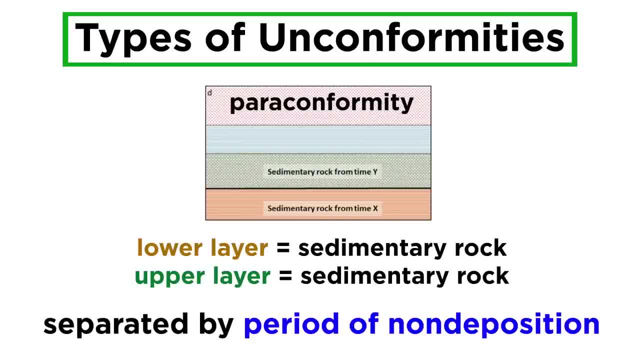 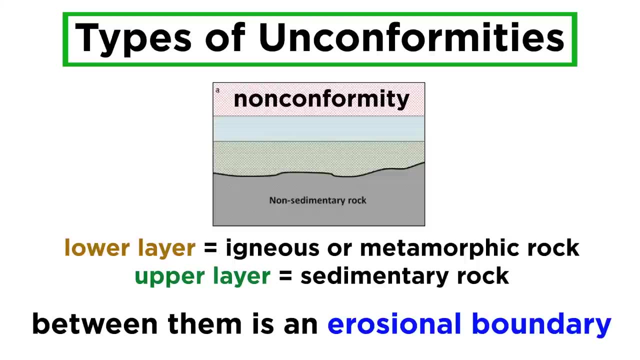 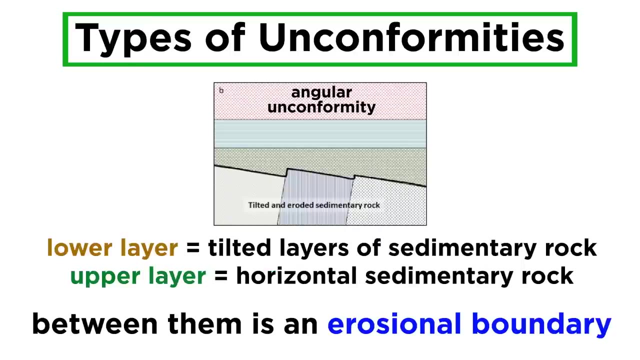 A paraconformity is also a boundary between two beds of sedimentary rocks, but is not erosional and simply represents a period of non-deposition. They represent less missing time than a disconformity. A nonconformity is a boundary between an older non-sedimentary rock, like an igneous or metamorphic rock, and younger sedimentary rock layered on top. And a nonconformity is a boundary between an older non-sedimentary rock, and an angular unconformity is a boundary between tectonically tilted layers of sedimentary rocks and overlying horizontal strata. 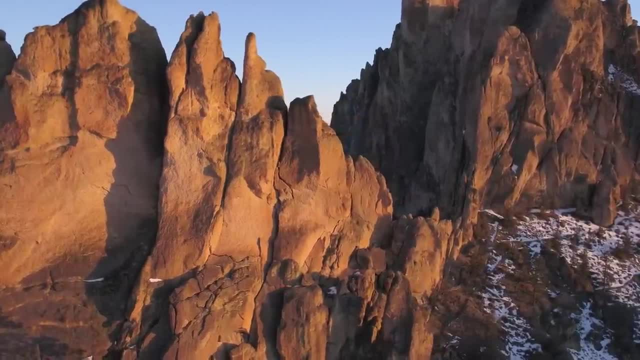 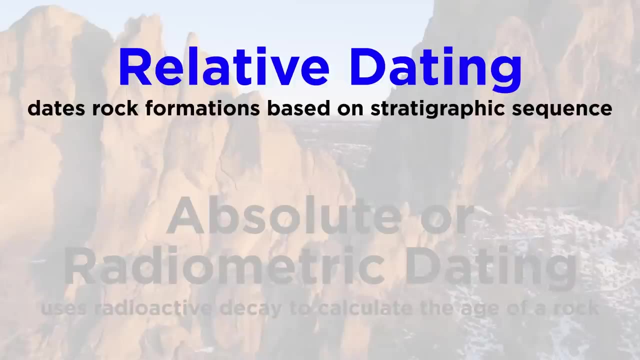 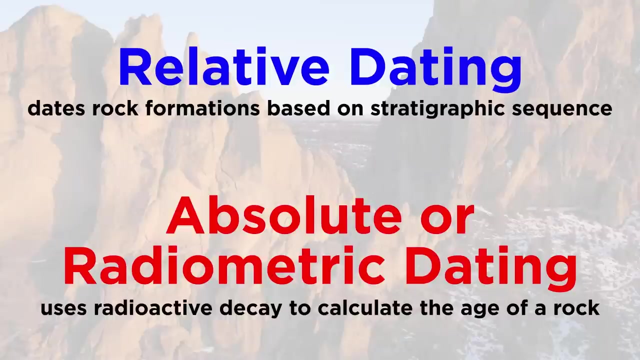 So that covers the principles that geologists use to assign relative dates to Earth's rock layers, and some of the challenges that this method poses. As we mentioned, prior to the development of radiometric dating, this was all that geologists were able to do, but radiometric dating is a powerful technique, so let's move forward and learn about that next. 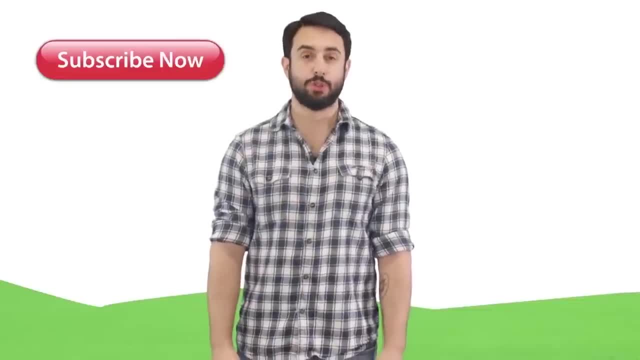 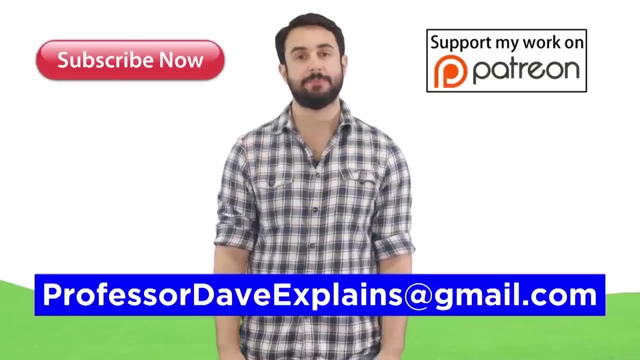 Thanks for watching. Subscribe to my channel for more tutorials, support me on patreon so I can keep making content, and as always, feel free to email me, professordaveexplains at gmail dot com. I'll see you next time!